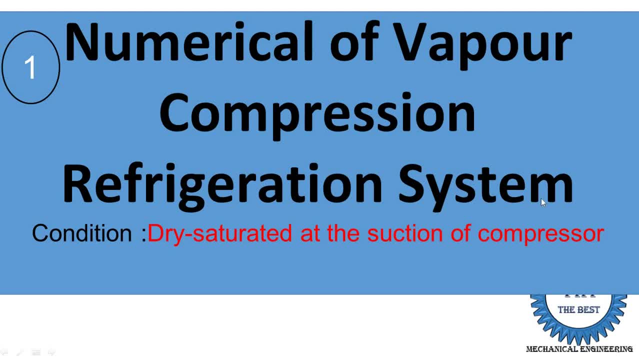 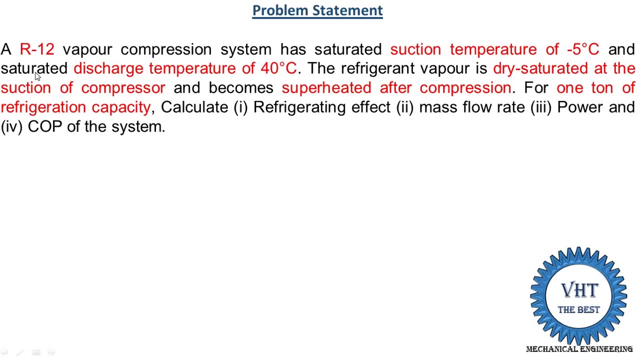 In this video I teach you the numerical of vapor compression refrigeration systems. and this is the example, type 1 or the problem 1, and in this the condition is given in the example is dry and saturated at the suction of compressors. So we move towards the problem statements. The problem: 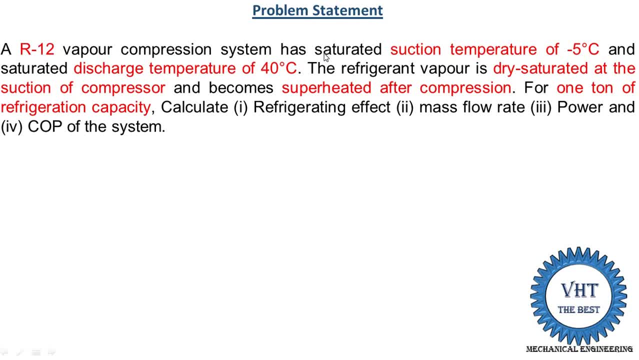 statement is that a R12 vapor compression system has saturated suction temperatures of minus 5 degrees centigrade and saturated discharge temperature is 45 degrees centigrade. That means the refrigerant in the system is R12. okay, So we use the refrigerant tables and pH content. 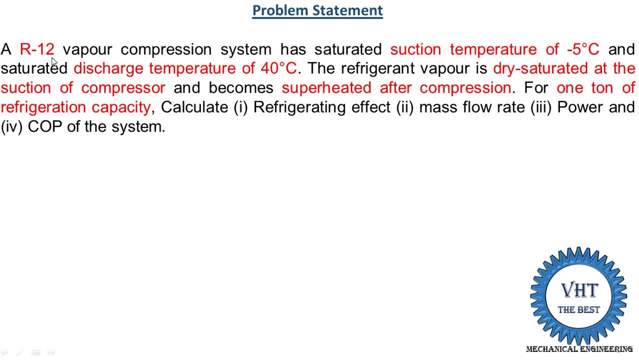 diagram for R12 refrigerants, because the pHché diagram is different for the different refrigerants and the suction temperature at the compressor is minus 5 and temperature of the refrigerant outlet from the compressor is minus 40.. The next given is the refrigerant vapor is dry and saturated. 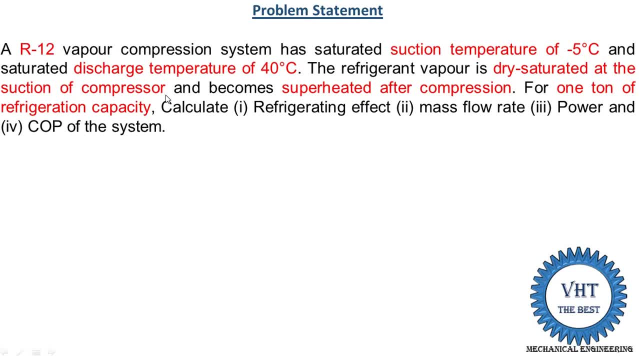 at the suction temperature of DΔav thread and Cth frequency temperature is minus 5. and with this I can conclude the paper fixed at saturation temperature at the compressor. at the of the compressor, that means at the inlet of the compressor, the refrigerant state is dry and saturated. that means point number one is: come on to the dry. 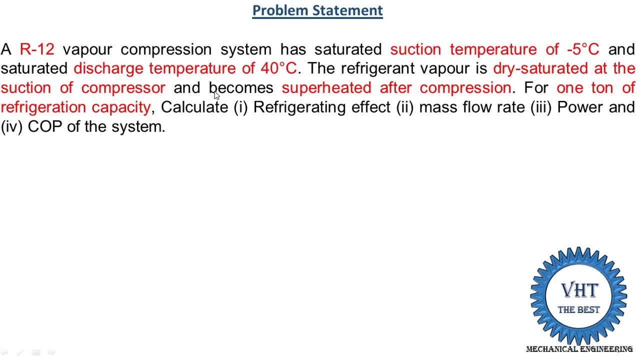 and saturation line or the saturated vapor lines, and become superheated after compression means point number two is given on to the superheated regions for one ton of refrigeration capacity. that means we considering that the refrigerant capacity is one ton and for one ton we find out all these calculation, that is. 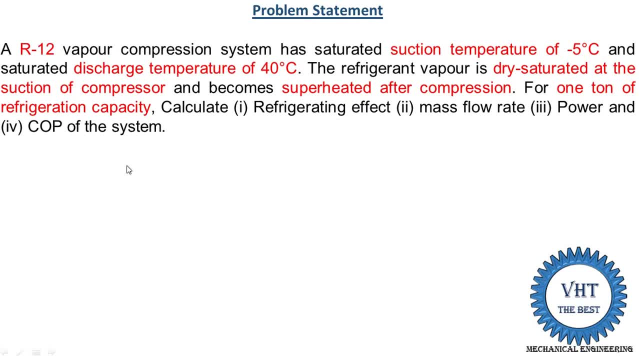 refrigerating effect, mass flow rates, power and COP of the system. so first we write down the given data. the given data is R 12 refrigerants. inlet temperature at the compressor, that is T 1 minus 5 degrees. centigrade outlet temperature of the compressor, or discharge temperatures is T 2- 40. 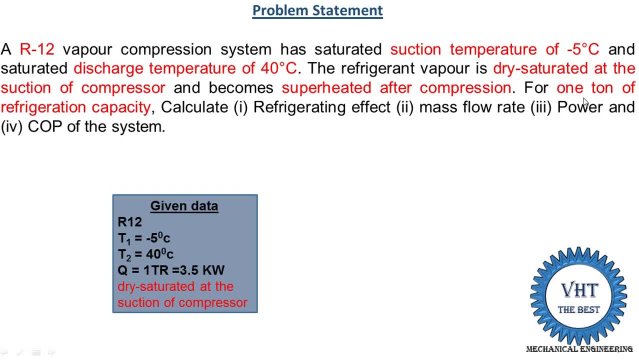 degrees centigrade and Q is equal to one ton, because we find out all the parameters for considering the one ton, and one ton is equal to three point five kilowatts. if you don't know how to convert the one ton into the three point five, one kilowatt, then the watch my. 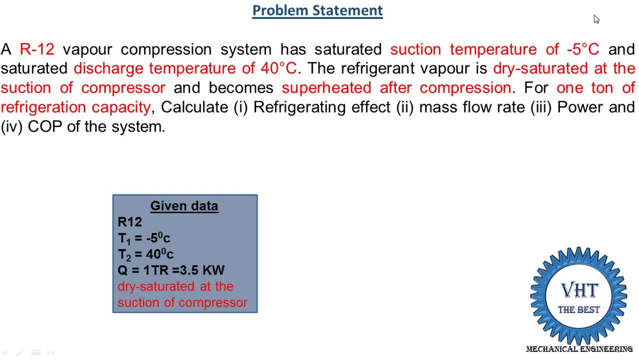 video on the one ton of refrigeration and link is provided on the top right screen and eye symbol and condition at the inlet of the compressor is given. that is a dry and saturated at the suction of the compressor. that means where to put the point number one. now what to find out? find out refrigerating. 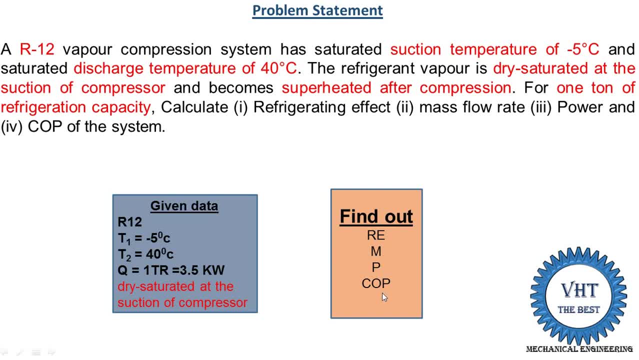 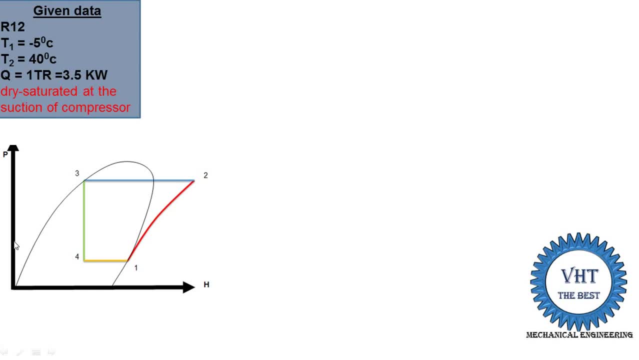 effect array, mass flow rate, M, power, P and the COP that is given. let's move towards the solutions, that is, the given data I already written here, and first draw the pH diagram to solve the examples. so this is the pH diagram of fesa system and, according to the given condition, food. 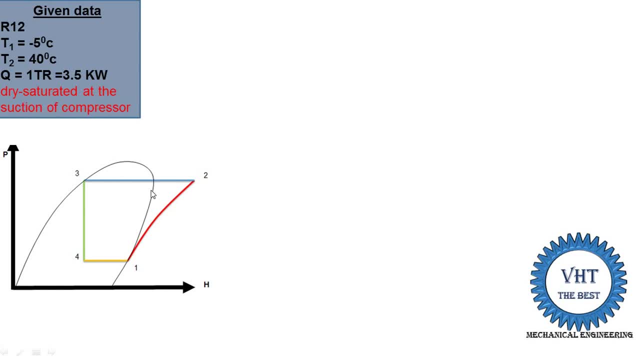 number 0.1, that is, a dry and saturated at suction of compressor. that means that means this is a critical point and from this critical point this is a saturated vapor line. so point number one is: come on the saturated vapor line. if you don't know how to put the point, then watch the my video on the pH diagram in. 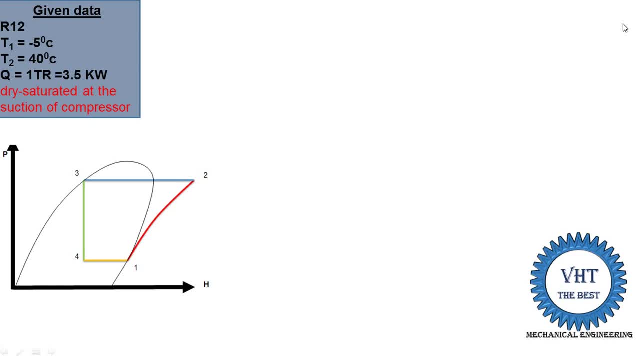 that you watching this video, you can understand how to put the points, that the point number one is on the saturated line, point number two in superheated regions, then three and four. is that okay? now for finding out this refrigerating effect, mass flow rate, power and COP we require to the enthalpy of that point. 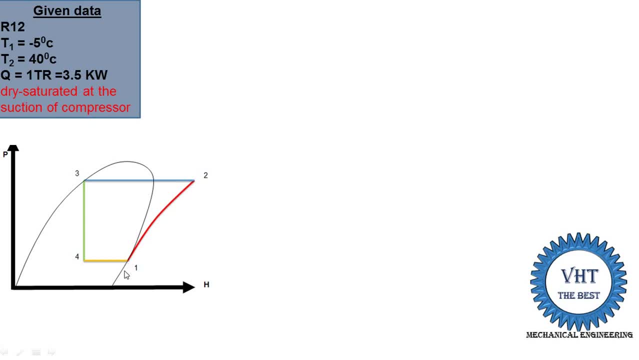 suppose we going to find out the work done, supplied to the compressor, so it is a one to two is compression process, that is h2 minus h1. but how to get the h2 minus h1, so which it is, find out from the table or the pH diagram. but in the 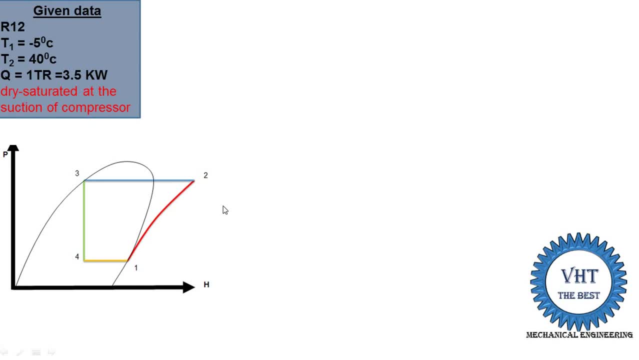 example, that is a compulsory to solve from the tables and you can only verify your answer of enthalpy from by using this pH diagram. so first we find out the enthalpy one by using the which table, that is, by using the r12 table, because 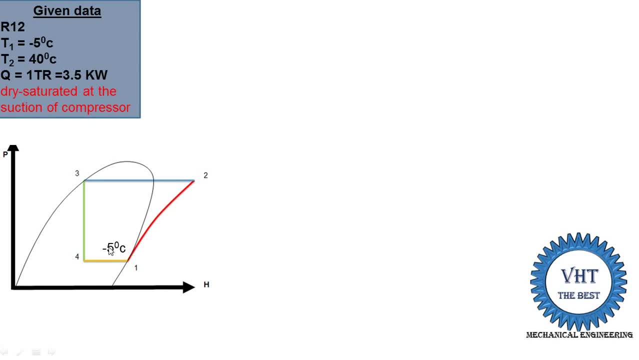 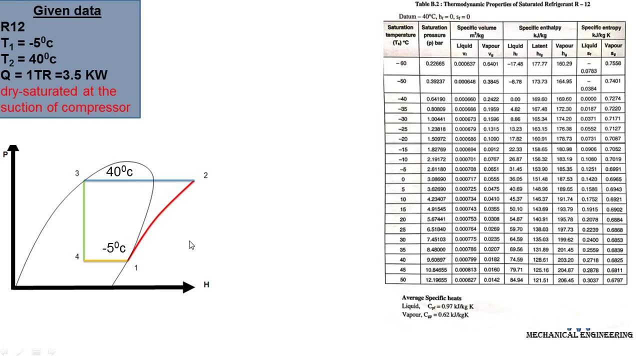 r12 refrigerant is given and first indicate this temperature at the evaporator minus h1, and then we find out the temperature at the evaporator minus five degrees centigrade and in the condenser it is a forty degree centigrade. so this is the refrigerant table r12. it is mentioned here on that. 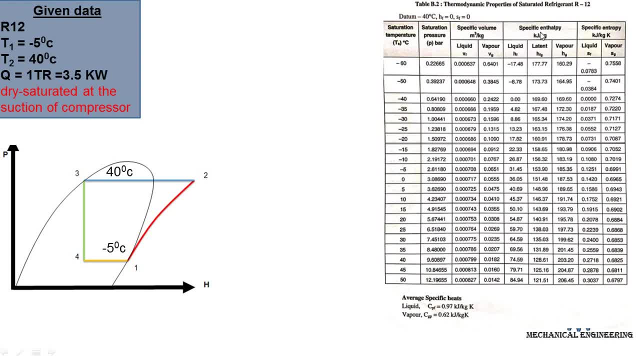 first is the temperatures, then saturation pressure, specific volume, specific enthalpy. enthalpy is given for liquid, latent heat and vapor. okay, and this is the specific entropy for liquid and vapor. so, point number one at the minus five degree centigrade, and a point number one, which is state of refrigerant. 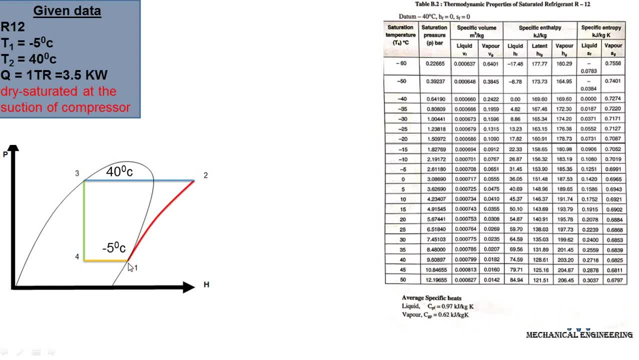 or vapor. it is a point. number one is on the vapor region. so we get the enthalpy of the gas or a vapor at the width temperature at the minus five temperature. so point number one is in minus five temperatures. so it is here the minus five temperature is given. so this box is for the minus. 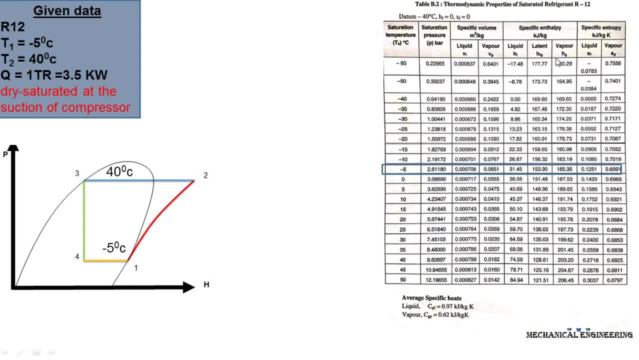 five. okay, and which enthalpy we take: hf, hfg or hd. point number one is on the saturation vapor line. that means gas. so we take the enthalpy for the vapor, hg. so hg is answer for minus five degree. centigrade is 185.35. now this value of enthalpy is different in the different table, if you using. 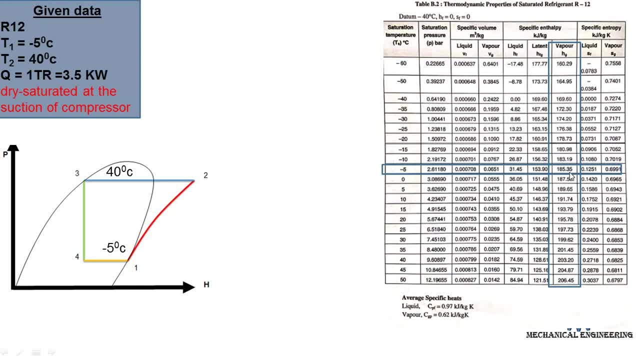 the different books, another books, then the enthalpy answer is different, but don't worry about that. your final answer is become same because we are subtracting the enthalpy, that is h2 minus h1. at that time your answer is correct. okay, in the different tables 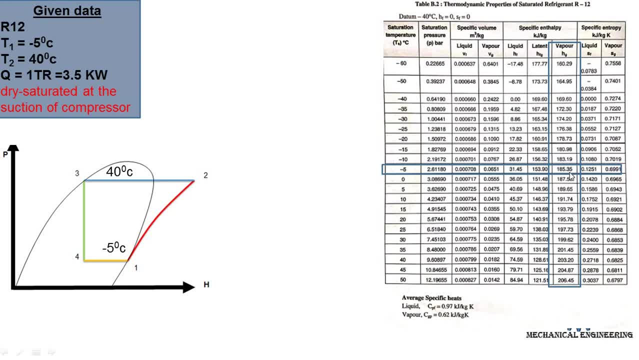 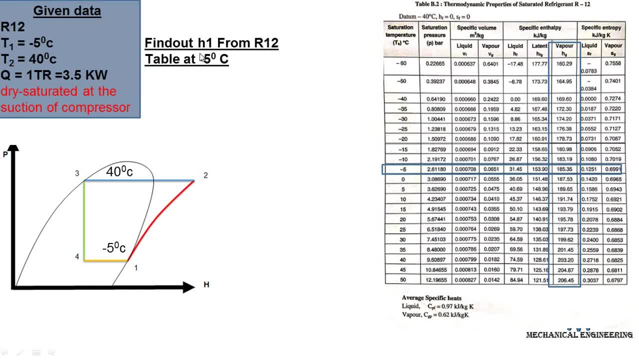 per kg. so from the pH diagram find out the h1 from r12 table at with temperature at the minus five. so read: the value of hg means h1 is equal to value of hg at minus five degree centigrade and value is 180.35. okay, next we find out the h2. now the h2 is not. find out from this: 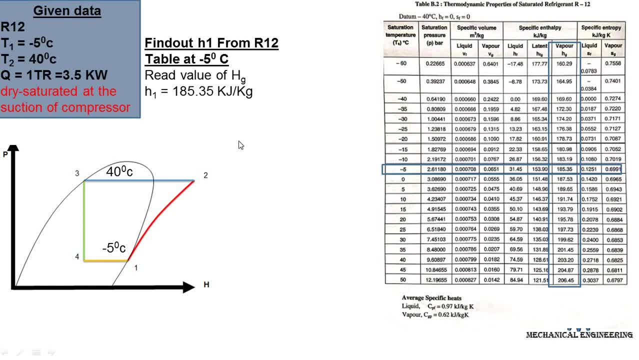 table because it is given the saturated, okay, but our point number two is on the superheated region, so for that we need to to calculate by using the different equations of the isentropic enthalpy, as s1 is equal to s2. okay, so first we find out the h3, now how to find out the. 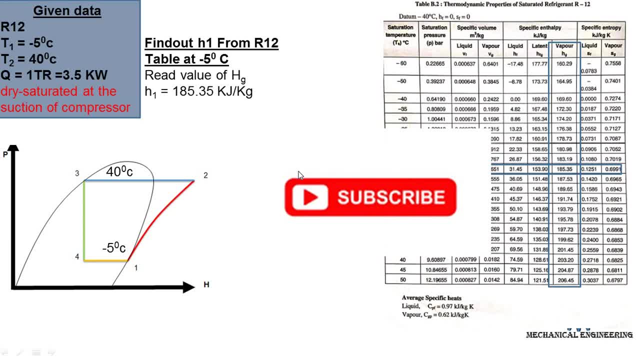 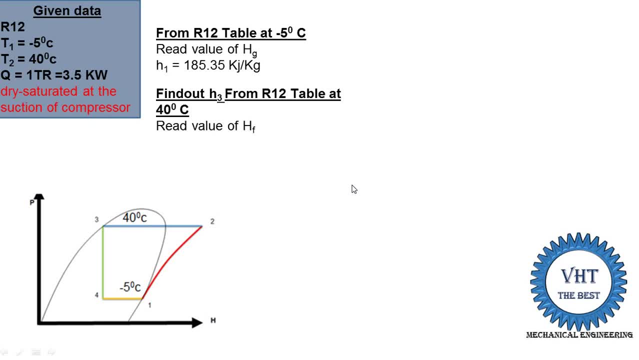 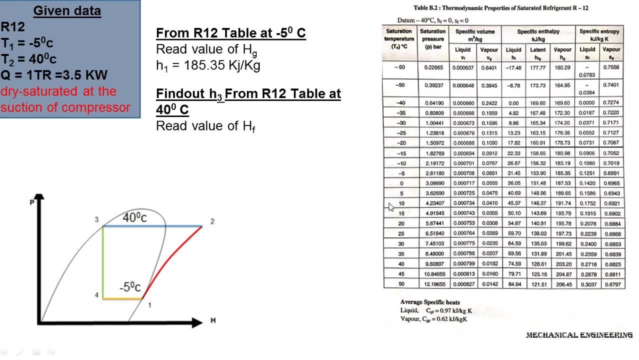 h3. let me see if you learn something. then subscribe my channel and like the video. and like the video now. next we find out the h3 by using this r12 tables for read. the value of hf means point number three is at with temperature, it is 40 degree centigrade, okay. 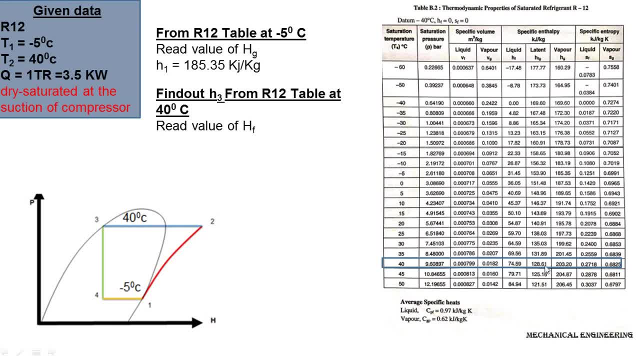 so we putting under rectangle here for 40 degree, and which enthalpy is considered. point number three is on the which region. it is, on the saturated liquid. so we take the enthalpy of the liquid, hf, okay. Number three is on the liquid region, so it is the hf. what is the answer? answer is h3. 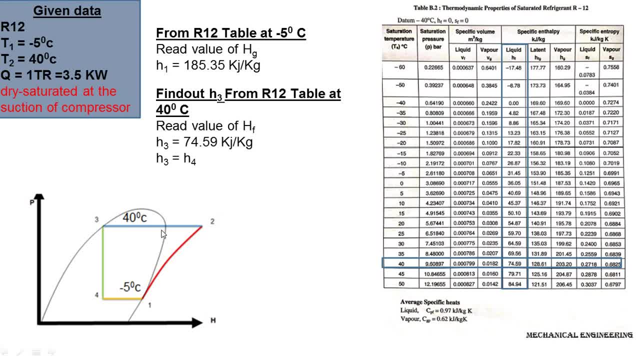 is equal to 74.59, okay, and h3 is equal to h4 because it is is a isentropic process. so h3 is equal to h4 and is equal to 74.59. unit is kilojoule per kg. again, I tell you that. 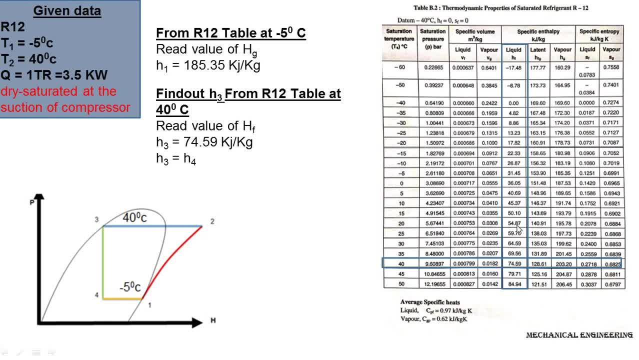 if your answer is different, because in the different books and the different tables, that is, a different answer is given for the enthalpy, but when we taking the subtractions the answer is different. The answer is coming perfect, okay, so don't worry about that now. next, if you learn something, 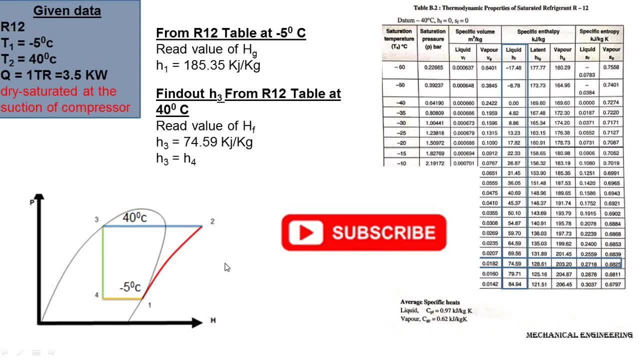 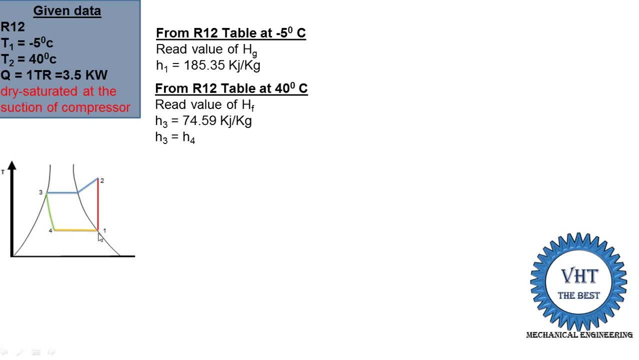 and like, then subscribe my channel for watching the more video and like my video now. next we find out the h2. okay, for one to two processes. which process? it is isentropic process. so for that process, so finding out the h2, we consider that s1 is equal to s2. okay, now how? 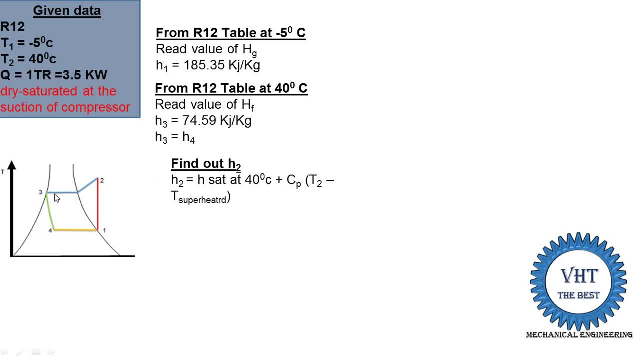 to find out the h2.. So we know the H2 value at 40 degree for the saturated vapor, okay, but point number two is the superheated. so we require to this temperature of the superheated vapor. so first we need to find out the T superheated. 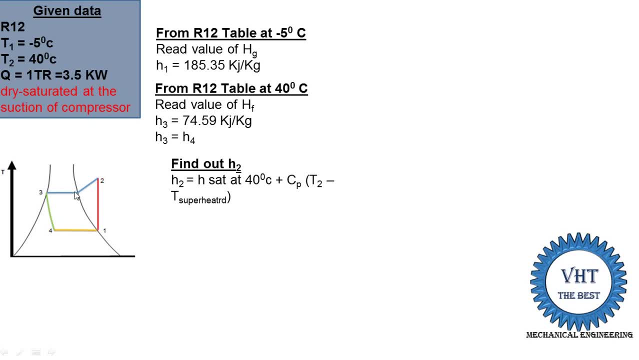 so h2 is equal to enthalpy at this saturated vapor plus Cp into T superheated minus T saturated. okay, so we need this. T2 is the superheated minus T saturated. Now we consider that isentropic process, s1 is equal to s2, so this is a t-s diagram, okay. 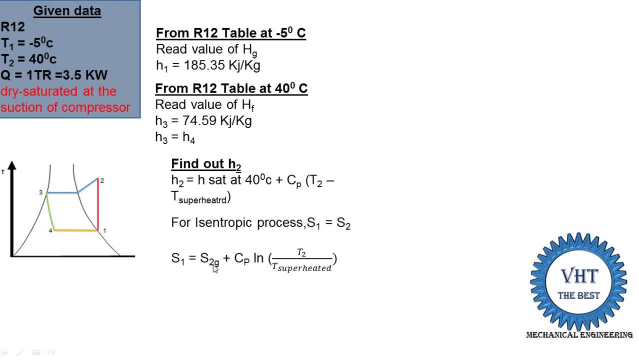 not the p-s diagram. so for, s1 is equal to s2g means at the point number two, that is a entropy for the gas means. at that point entropy is given in the table, not this point. entropy is given plus Cpl n, T2 upon the superheated. this is the standard equation for finding out. 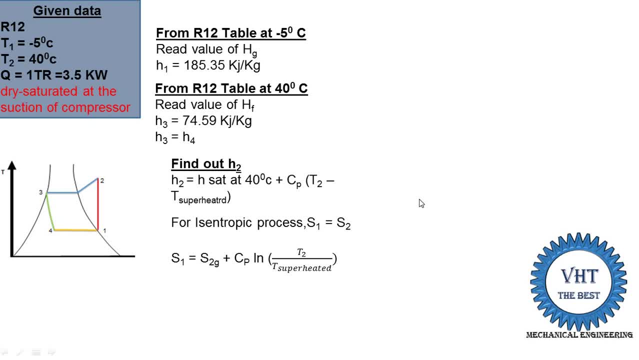 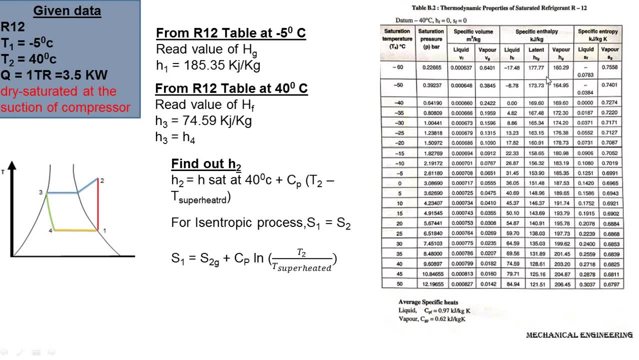 the T superheated For, for the superheated region. so for that s2g, s1 is not given, cp is not given, so for that we need to the table of r12. ok, so first we find out the value of s1, then s2, cp, and by 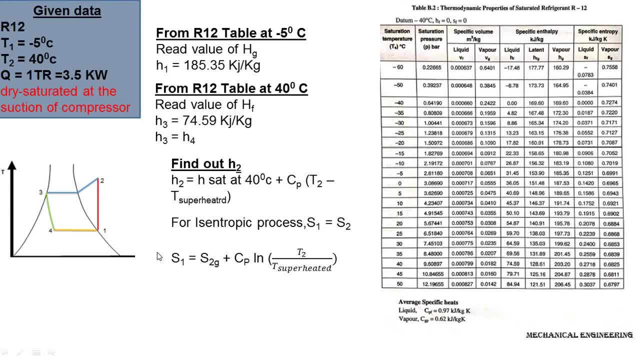 putting this value, we find out the t superheated. so what is the value of s1? so s1 is at the minus 5 degree centigrade. ok, and minus 5 degree centigrade, which is the state is gas, ok, so here the minus 5. so i put one rectangle here and this entropy is this side, that is a specific. 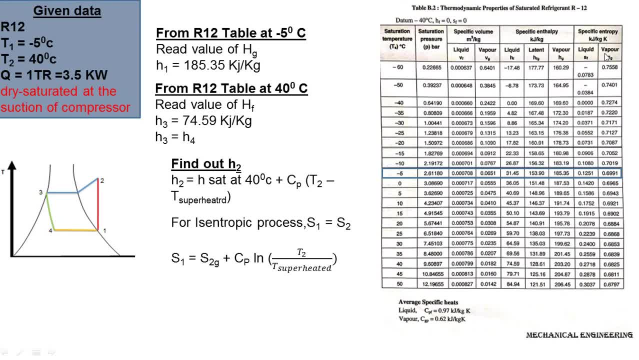 entropy unit is kilojoule per kg. 2 entropy is given for liquid or vapor, which we take. point number was in the vapor region. so we take the entropy for the vapor. that is a sg and the value is 0.6991 kilojoule per kg kelvin. so here we write down that s1 is equal to: 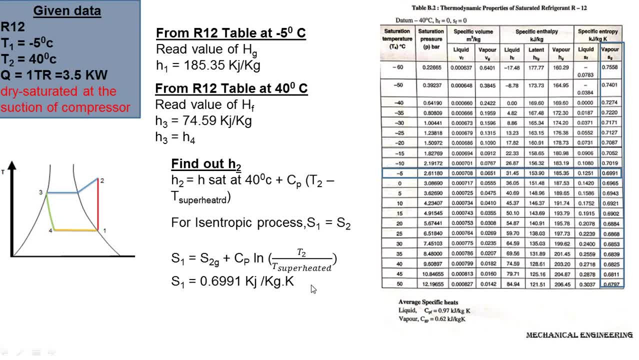 0.6991 kilojoule per kg kelvin. if your answer is different, don't worry about it, because it is different. unit is there, but final answer of t- superheated is same. next we find out the s2g means. two point is at the 40 degree centigrade. so we coming here at the 40 regions. 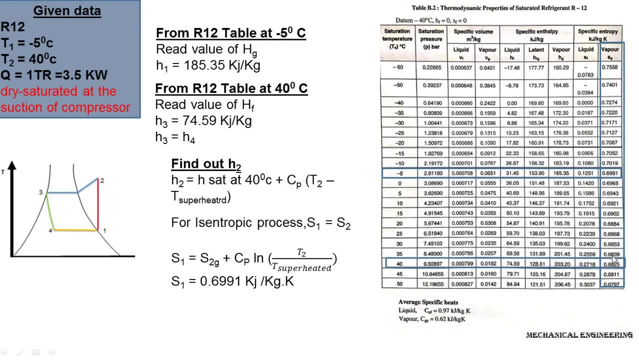 it is also the vapor region, so we take the vapor entropy. that is a 0.6825, so s2g is equal to 0.6825. unit is same. that is kilojoule per kg kelvin. next is the cp. that means specific. heat is given by the vapor. that is 0.6825. so s2g is equal to 0.6825. unit is same. that is kilojoule per kg kelvin. next is the cp. that means specific heat is given by the vapor. 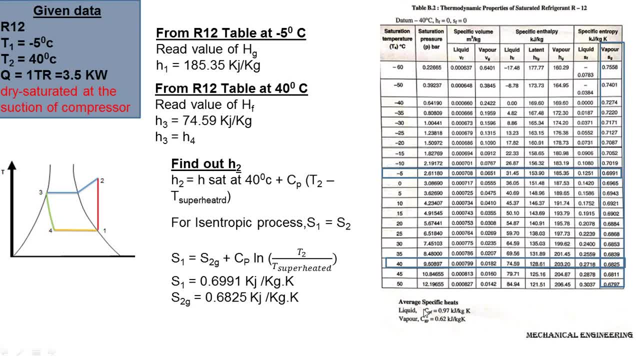 so specific heat is given here in this table, specific heat for fluid or gas. so we take for the vapor, because point number one is on the vapor region, and this specific heat, cp is equal to 0.62 kilojoule per kg kelvin. now we putting this value on this equation. 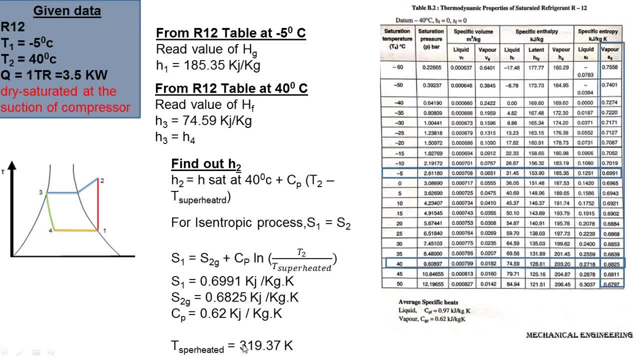 and we find out the t superheated and t superheated is coming in the kelvin because the all the entropy and the cp is on the kelvin and we also put this t2 in the kelvin, that is a 40 degree centigrade is given, so value. 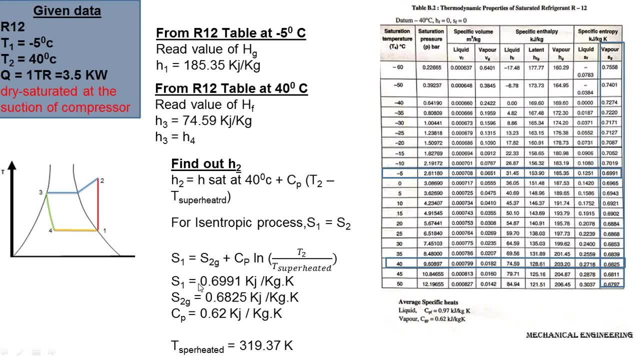 of the t2 is put at 313 kelvin because the s1, because entropy and specific heat, is in unit of the kelvin, because kilojoule per kg kelvin. so put the t2 in the kelvin and we get the answer of t- superheated, is 319.37 kelvin. now we putting this value on this equation. 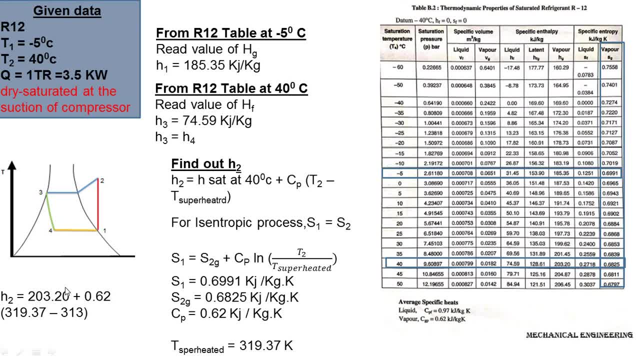 of the h2.. so h2 is equal to 0.6825.. h2 is equal to now. for that we take the enthalpy at the 40 degree centigrade, that is a 203.20. for that it is a 40 degree, and take the enthalpy of the vapor, it is a 203.20. ok, plus cp is 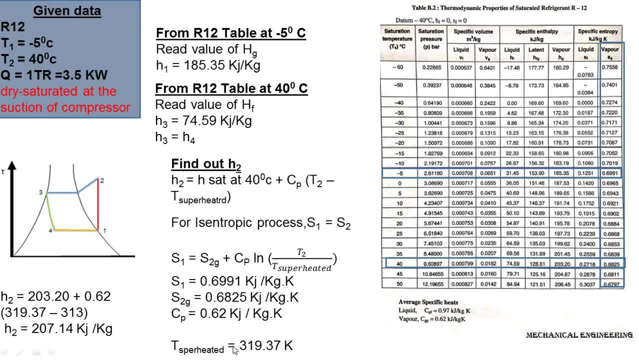 0.62. t superheated is 319.37. minus t superheated is 319.37.. ok, t2 is the 40 degree, means 313 kelvin. so h2 is equal to 207.14 kilojoule per kg. now we 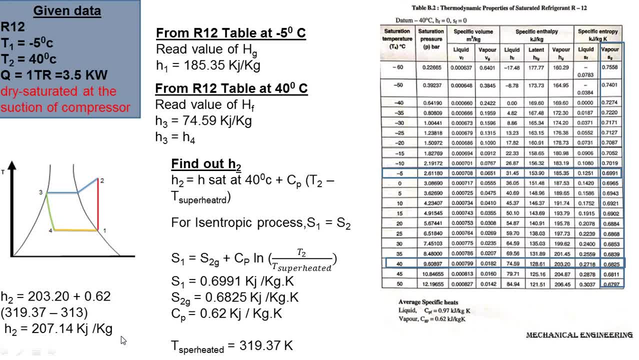 have all the enthalpy: h1, h2, h3, h4. now this is the only complicated things to find out the all enthalpy then after the example is too easy, numerical is too easy to calculate. ok, because it only consider the difference of enthalpies. now, if you learn to something, 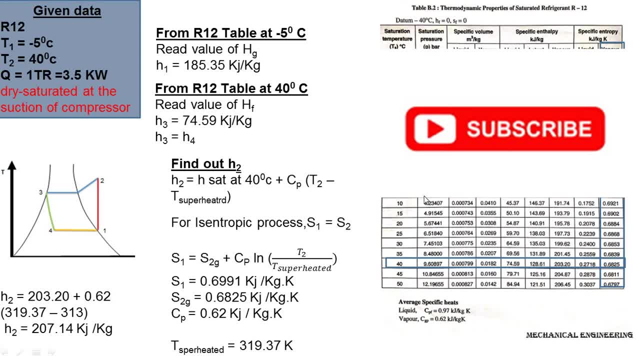 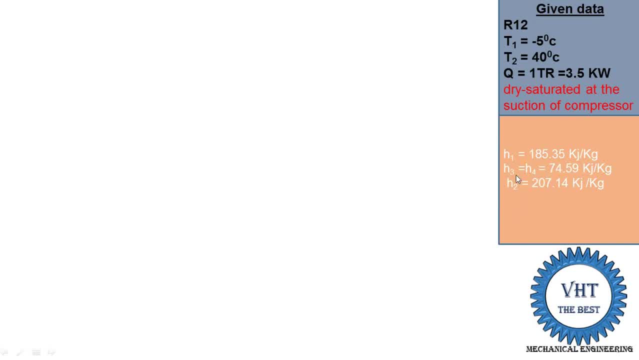 and how to find out the enthalpy and entropy. then subscribe my channel to watch more videos. bye, bye, now I return here. all the answer of h1, h2, h3 and h4. ok, so we can easily putting this value now. first we find out the refrigerating effect. what is the answer you need? sorry equation. 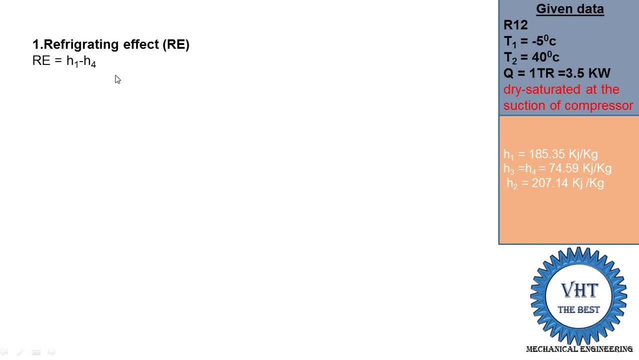 for refrigerating effect. it is h1 minus h4. this refrigerating effect is produce into this evaporators. ok, so it is in. the evaporator process is 124, so it is h1 minus h4. now we have the value of h1, we have value of h4 that is put at h2.20.40.. 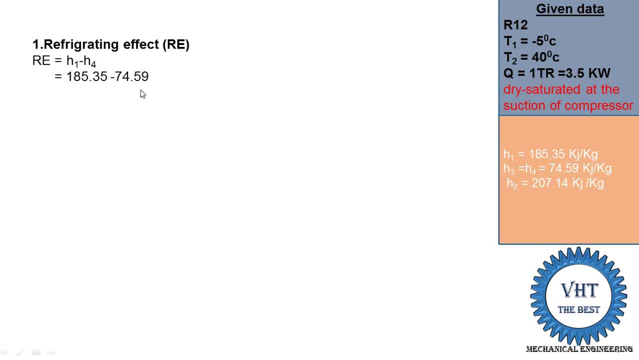 Now, as per say, temperature could be mudar the temperature. it is put that h1 is equal to 185, point 35, h4 is equal to 74.59. ok, so we do that and answer it: 110.76 unit is kilojoule per kg, because enthalpy is in kilojoule per kg. next we find: 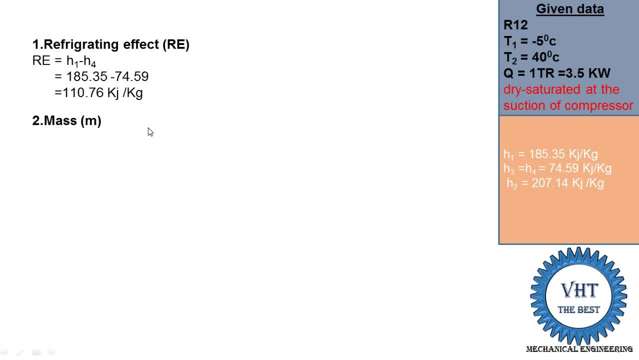 out the mass flow rate. now, all this thing is find out for the 110, because in the exp извereens thinkmeed it is mention. then find out for the 110 of the capacity. ok, so for broadcasting, so for mass is find out for the mass. m is equal to q upon h1 minus h4, because this is a 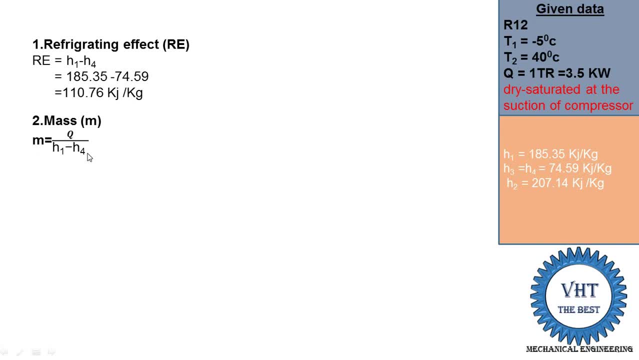 refrigerating capacity. q is equal to m into h1 minus h4. from that we make the m to find out: and m is equal to q upon h1 minus h4 and q is equal to given one ton, and one ton is equal to 3.5 kilowatt. 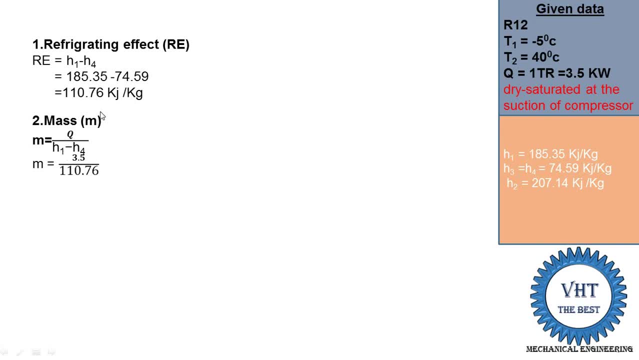 so q is equal to 3.51 h1 minus h4 already done here, that is a 110.76.. So we get the answer. of m is equal to 0.0315 kilojoule per second. Now how to know this unit? because the q in the unit is: 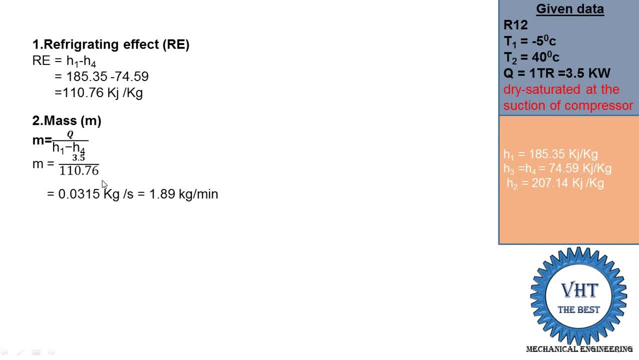 kilowatt, that is kilojoule per second, and this h1 minus h4 is kilojoule per kg. so kilojoule, kilojoule is cancelled. kg is going on upper sides okay, and the second is coming downward side. weight is kilogram per second. then we multiplied with the 60, then unit is come in the 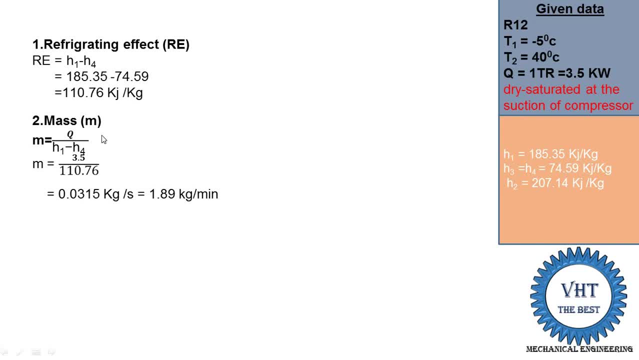 kilogram per minute. so you just put the unit of q, that is kilojoule per second, in the downside. you put the kilojoule per kg, okay, and you get the answer. unit answer is the kilo kilogram per seconds. then we find out the power. so power is equal to. that means power is supplied to the 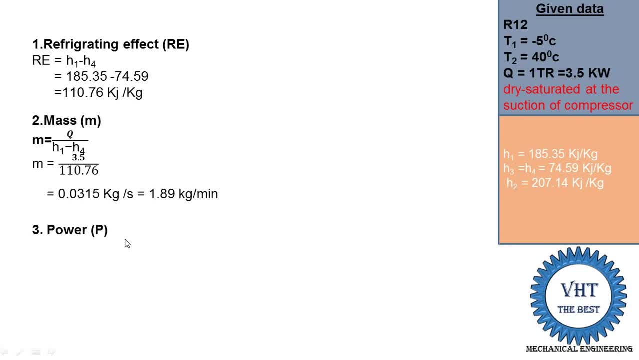 compressor in compression process is the 1 to 2, that means power is equal to h2 minus h1. okay, and it is multiplied with the m, then power is find out in the kilowatt. okay. now if we only consider h2 minus h1, then unit is kilo kilojoule per kg. but we require to find out the power in kilowatt. 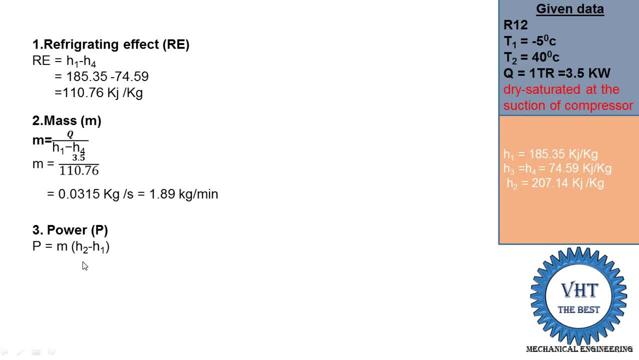 that is kilogram per second. that's why here it is multiplied with the m, so m is equal to 0.0315, h2 is equal to 207.14, minus h1: 185.35. okay, so here unit of mass is kilogram. 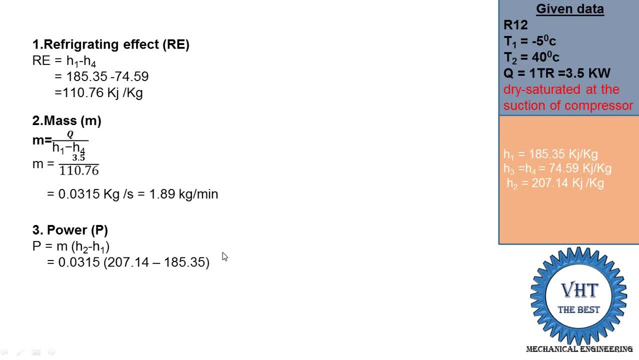 per second into enthalpy unit is kilojoule per kg, so kg kg is cancelled and unit for the power is come kilojoule per second. or kilojoule per second is equal to kilowatt and answer is 0.68 kilojoule.